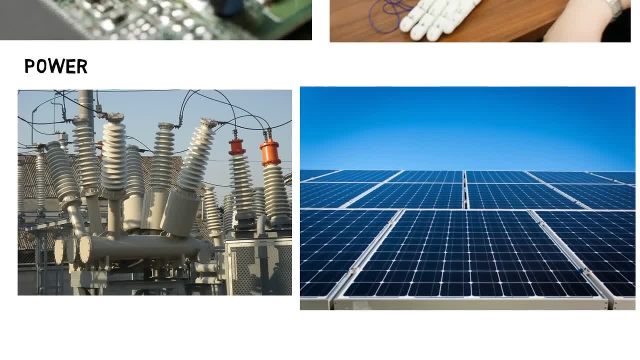 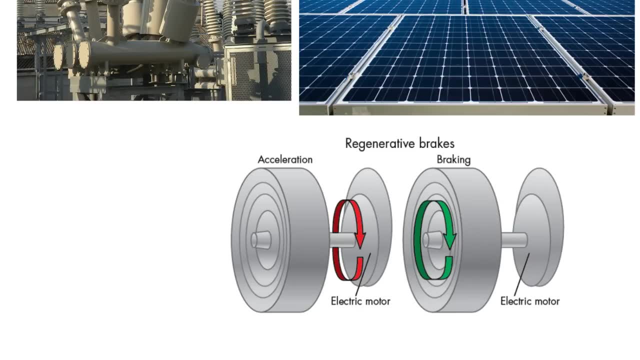 at a power plant working with solar panels or something like electric motors and regenerative braking where, like in certain electric vehicles, when you take your foot off the accelerator, the motor turns into a generator due to changing speeds of certain components within the system. 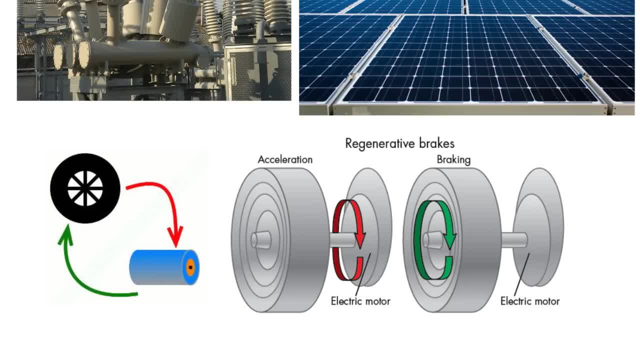 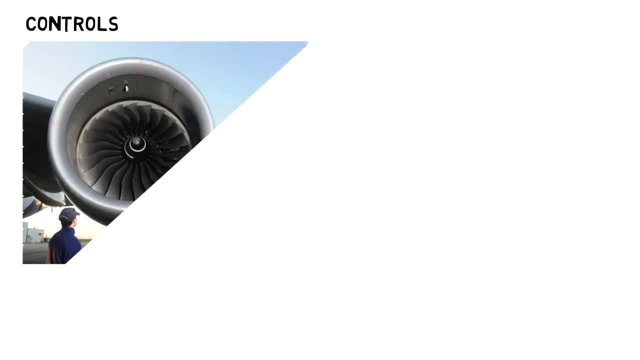 and then the kinetic energy of the wheels is used to generate electricity that can be stored for later use. There's controls where you'd work on things that have some sort of electrical feedback, like propulsion systems in various aircrafts all the way to your. 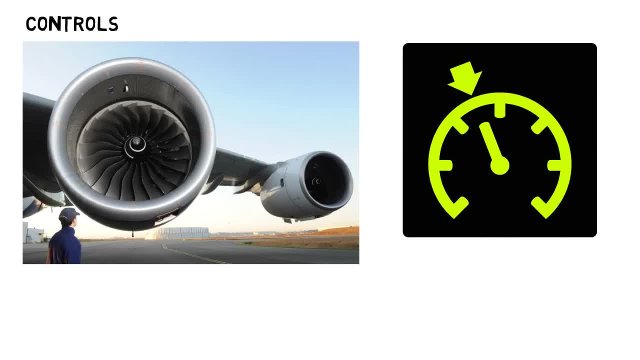 cruise control, where your speed is monitored. then, depending on what it receives, the system turns the wheels faster or slower accordingly, which then affects your speed, which is then fed back into the system, and this control loop continues. There's instrumentation. 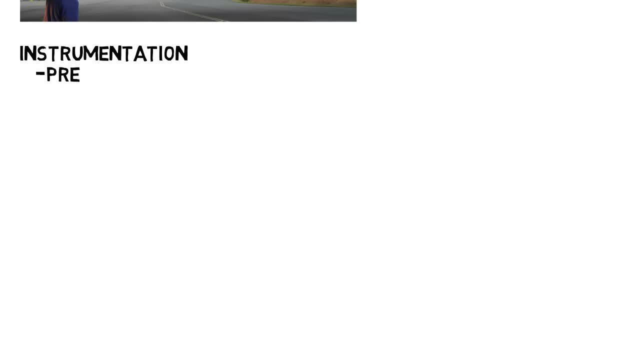 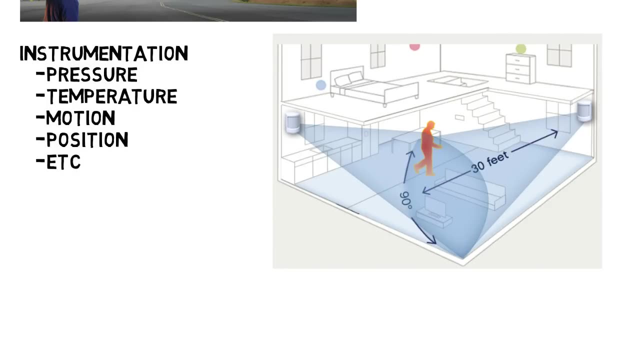 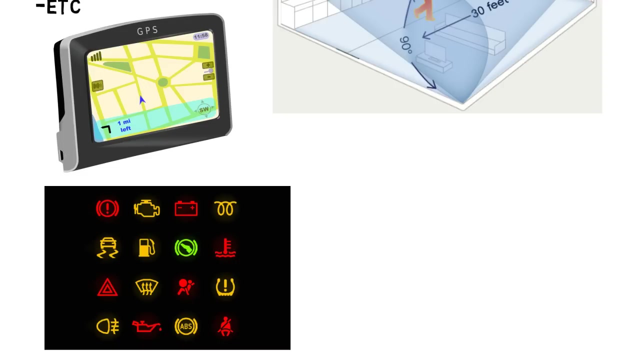 which deals with designing sensors and equipment to measure physical quantities like pressure, temperature, motion position and so on. You could design motion detection sensors for a security system, GPS for aircrafts or all the sensors in your car that have to analyze fluid levels, temperatures, battery voltage, anti-skid braking system or more. 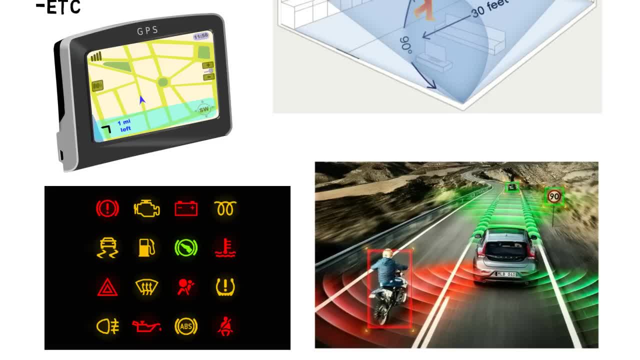 advanced systems for driverless cars. These types of electrical engineers often work with controls engineers, because after all, a controls engineer could design a great system to control the speed of an aircraft, let's say. but if all the sensors cannot accurately determine the speed, air pressure and so on, 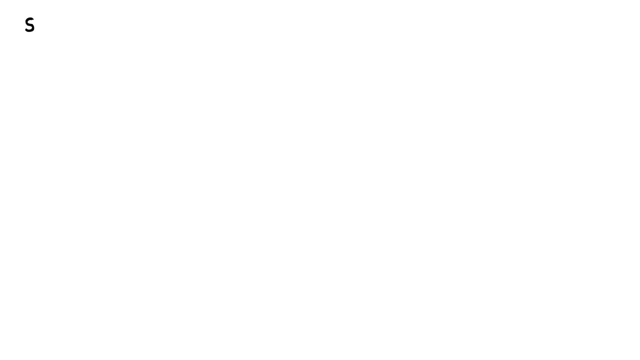 the control system is basically no good. There are many of these fields, but the last one I'll explain is signal processing. This is simply about the manipulation and analysis of signals, Signals being essentially functions that convey some sort of information. Maybe you have this sinusoidal voltage at some frequency. 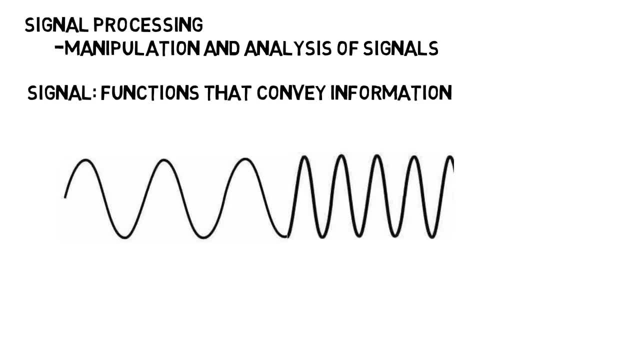 and then a sensor in the system causes an increase in the frequency and that frequency change is related to the temperature that the sensor is picking up. Now that changing voltage or signal contains information about the temperature in the room that we could convert to text on a screen, let's say. But when it comes to signals in general, you might 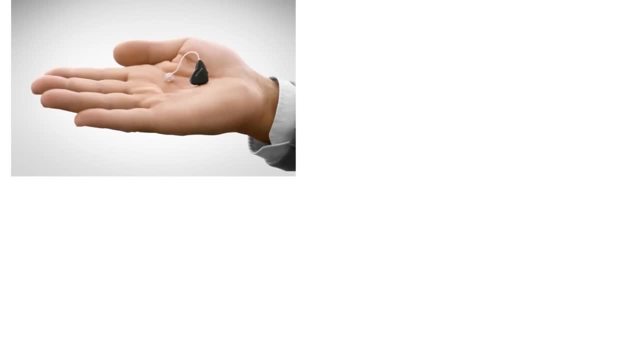 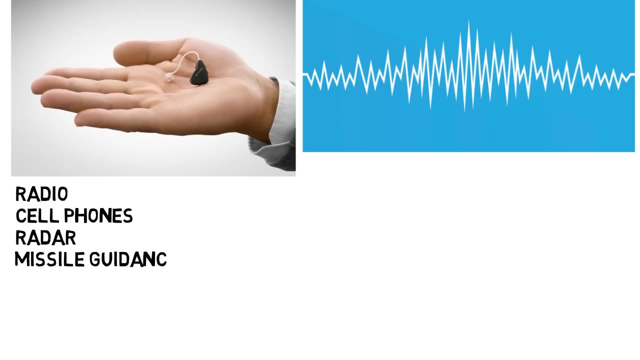 have to amplify them, like for an earpiece, or filter them where there's background noise and much more, And this can apply to radio signals, cell phone signals, radar, missile guidance systems, speech, image or video processing. This can be applied to radio signals. 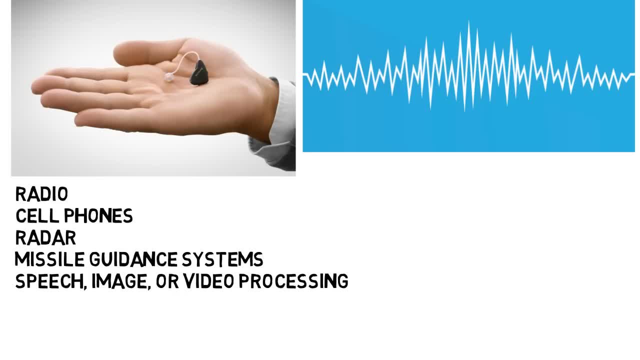 cell phone signals, radar, missile guidance systems, speech, image or video processing. That all involves signals that need manipulation. There's GPS signals, noise cancelling headphones and, of course, way more. Okay, now I've already thrown a lot at you to encompass a lot of what you can do as an 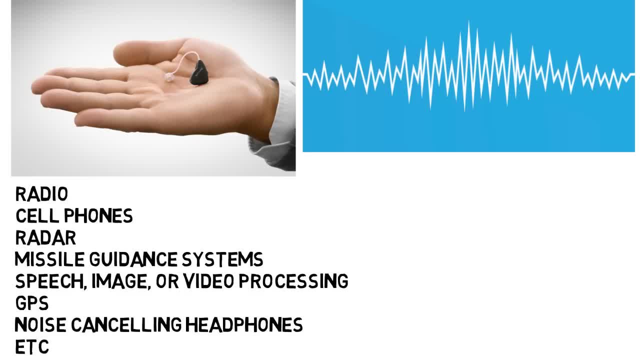 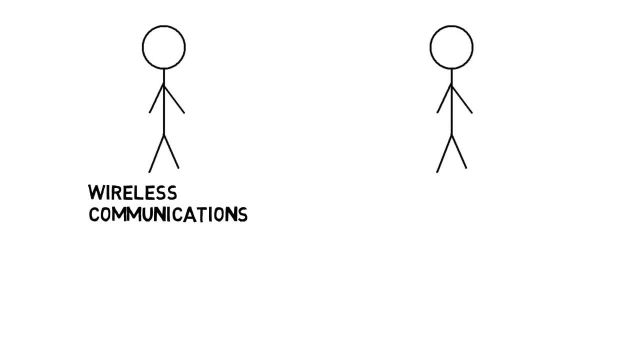 electrical engineer and, as you can see, it's very broad. it's not just one thing, As in, two people who majored in electrical engineering, as with many other engineering disciplines, could be in two totally different fields or careers and have very little knowledge about. 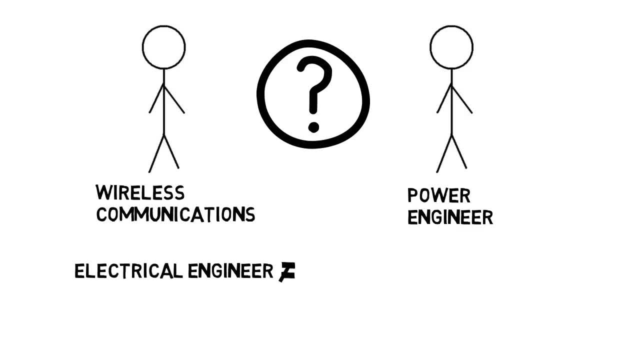 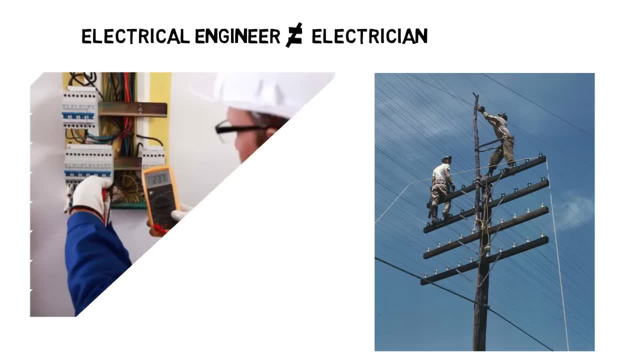 each other's work. And this is also not about being an electrician, by the way, which is a common misconception- Not where you go in and install or repair electrical systems in people's houses or offices and so on, But if you're debating, picking this as a major, all the fields I've discussed 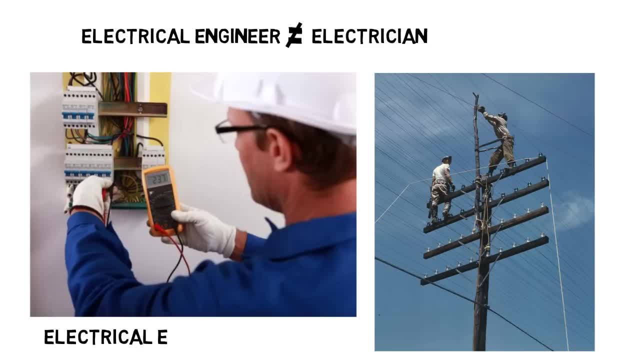 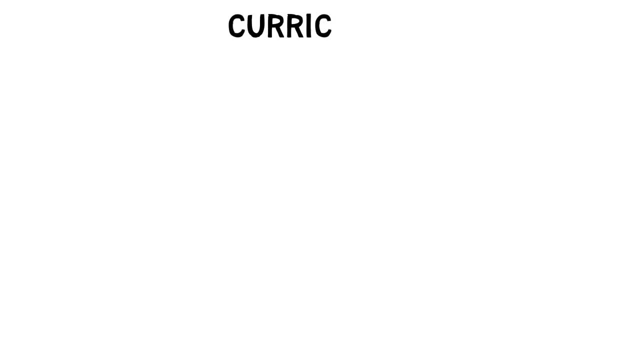 could seem like a lot and you may be thinking: wait, what does an electrical engineering major look like and what can I expect? and that's what we'll go into now. While all schools are a little different, a typical electrical engineering curriculum consists of a few circuit analysis classes, to just get you started. digital design, a. 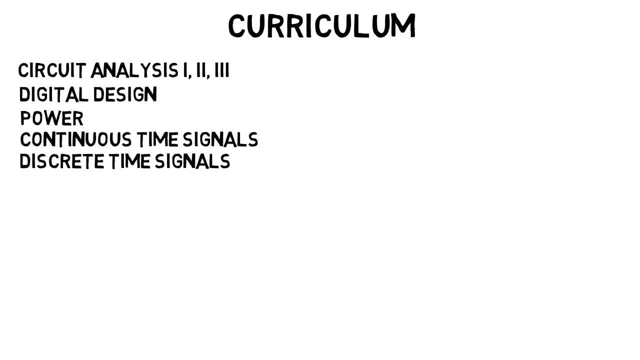 power engineering class, continuous time signals and discrete time signals, which are what get you started with electrical engineering and electrical engineering as a major. And you'll take a controls class, a communications class which you'll learn the basics of FM and AM radio, a basic electronics class which likely is followed by analog and digital electronics. 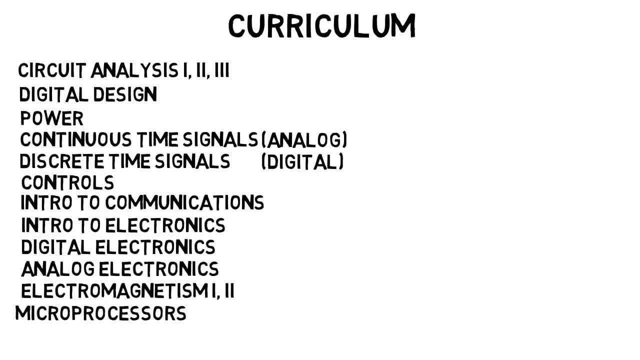 some electromagnetism courses, which are basically physics classes and a microprocessor class. There are some others you'll take and this doesn't cover the math or physics classes that you'll see, but these are the big major classes to expect in undergrad, Don't worry. 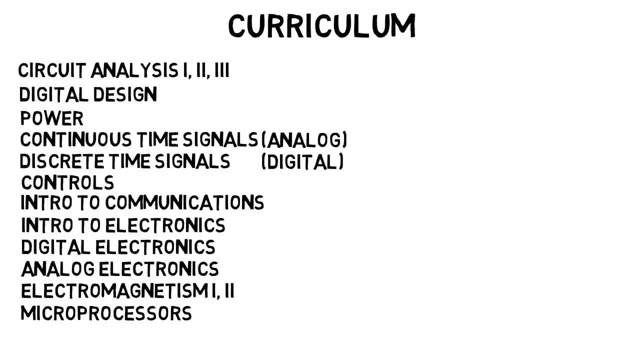 about what they are for now. but just know this is pretty typical. Now see how, regardless of who you are, you'll take some classes on most of those sub-disciplines I mentioned earlier. You got your power class. you got some signals classes, wireless communications. 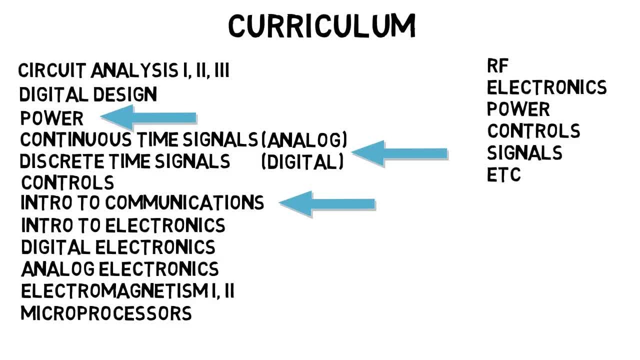 controls and so on. As an undergrad you get exposure to a lot of foundations of electrical engineering and you become well-rounded, but you don't become an expert in really any field. That's where masters and PhDs come in, or just simply working in a field. 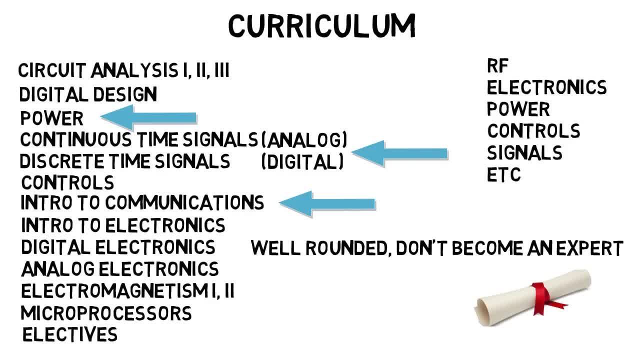 for many years. of course, You will be taking electives in the sub-fields you're most interested in, though, towards the end of college, so you will gain a little more mastery in those classes, which diversifies you and your resume from others, but it's not the bulk. 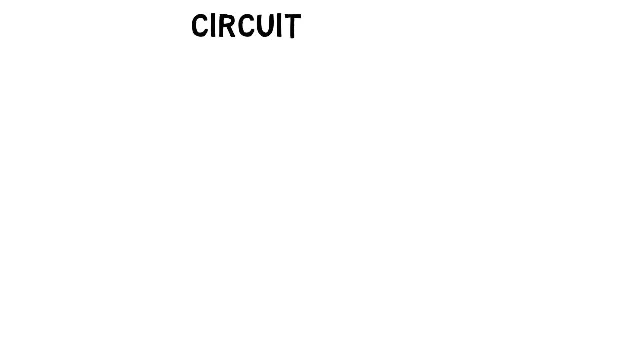 of your curriculum. But now let's go through these a little. The first are the circuit analysis classes. Now, if you've taken physics classes in high school, maybe you've seen the basics of resistors, capacitors and inductors And you're going. 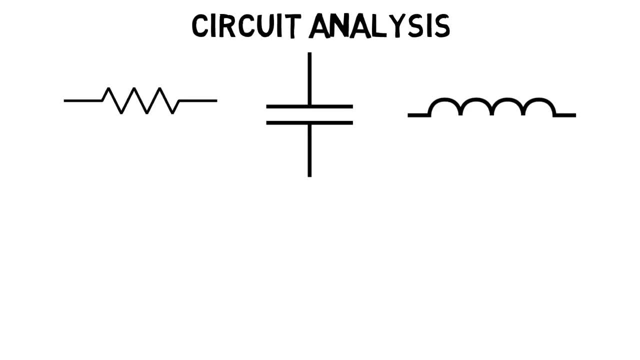 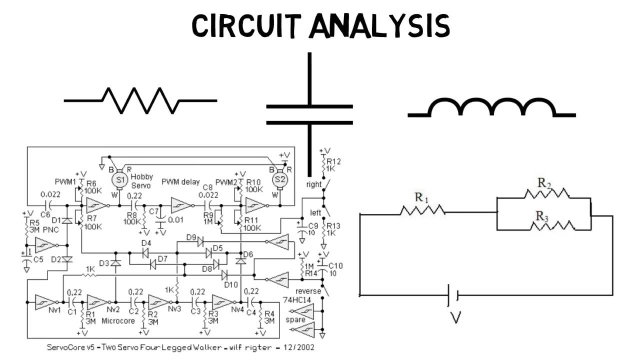 to learn how to find the voltage and current in circuits that contain these three components, first starting off with just resistors, though In the real world circuits are normally extremely complex. But in school you've got to learn the basics of voltage and current in a circuit. 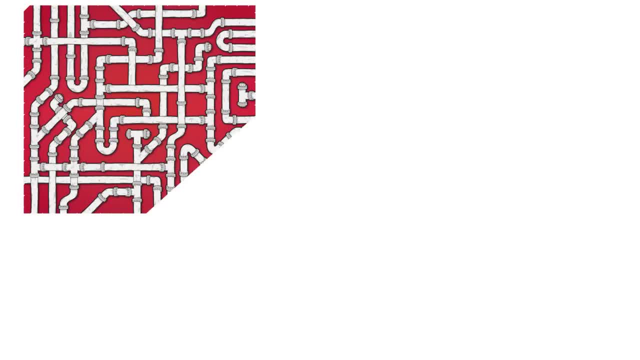 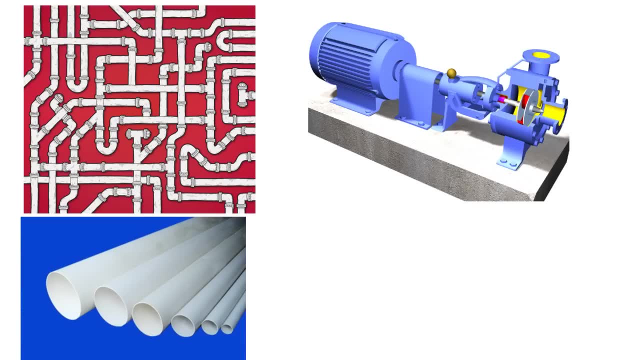 For those who may be unfamiliar: if you imagine a network of pipes, you could use a pump that creates a pressure difference and causes water to flow around and through all the pipes. If the pipes are skinny, let's say, it'd be harder for water to flow through them. 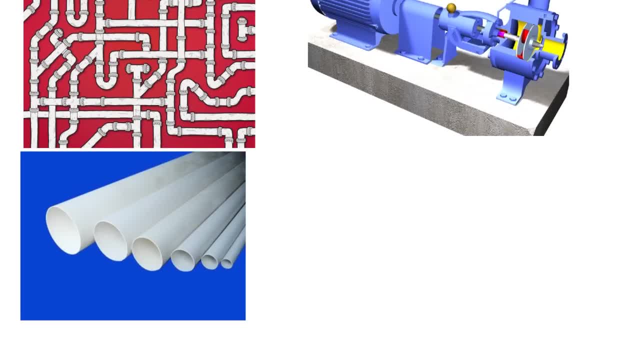 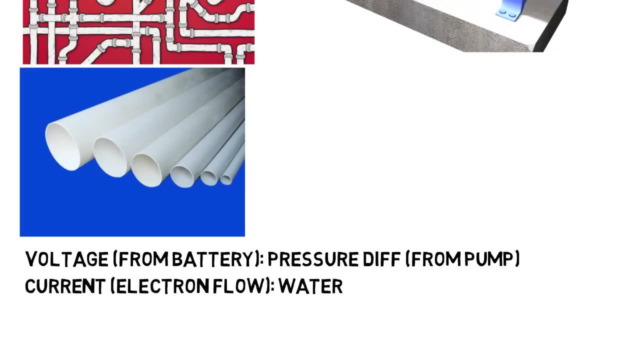 And if they're thicker then of course it'd be easier. Well, in a circuit, the voltage from, maybe, a battery is like the pressure difference from the pump. The current or electron flow is like the water And the resistors are like 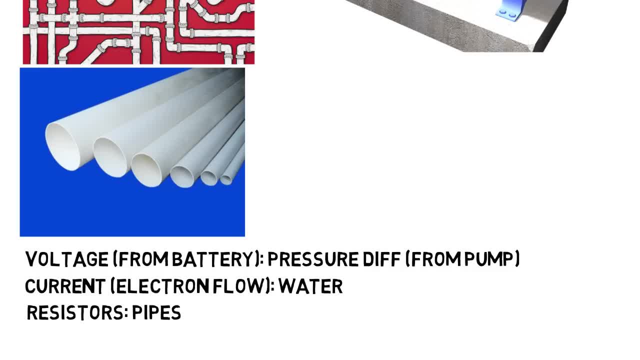 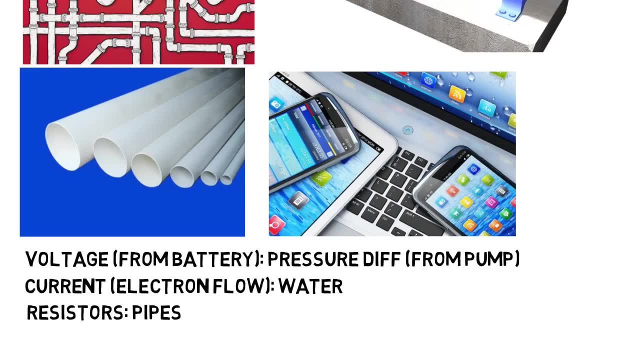 the pipes harder for water or the current to go through. Your electronics work for many reasons, but mainly it's because electrons are flowing through the device. In school you learn techniques to find the voltage difference across various resistors, just like there'd be some pressure difference across each. 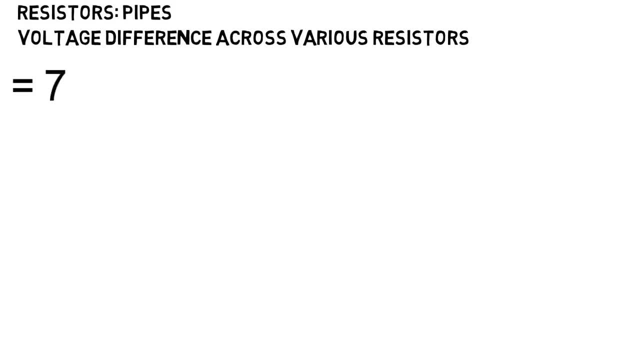 individual pipe Circuits. classes are a lot of systems of equations, just like you learned in school before, but more variables. usually, instead of X and Y, it's usually V and I for voltage and current And to begin all the circuits have a constant voltage as an input, like a 9 volt battery. that is not changing. 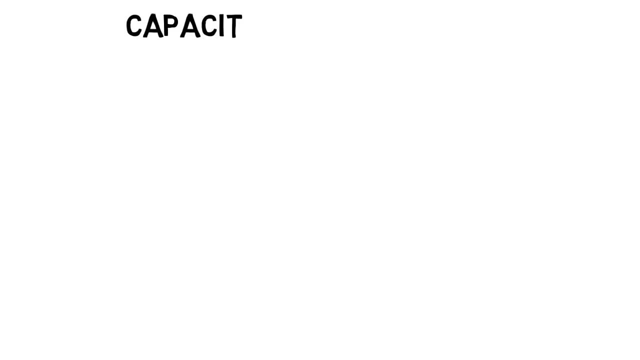 Then in the second level circuit analysis class you get into capacitors and inductors. You'll use those same circuit analysis techniques and the voltage source will still be constant, like a battery, but current and voltage in the circuit across those components change in an exponential way, like 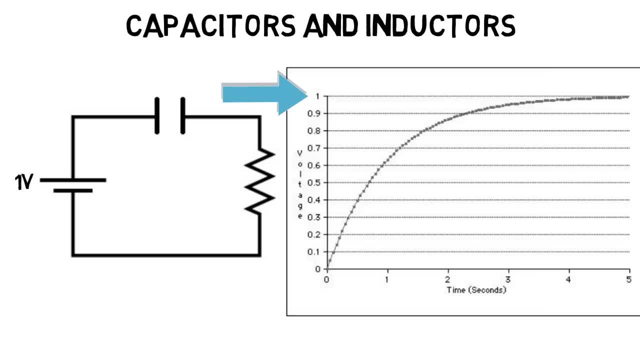 charging up a capacitor to a max voltage. In order to find that max value, or the time it takes to charge up to, let's say, half the max value, you will use circuit techniques to find the resistance in the circuit, and so on. Then you'd quickly move on to AC circuits or alternating current, where the 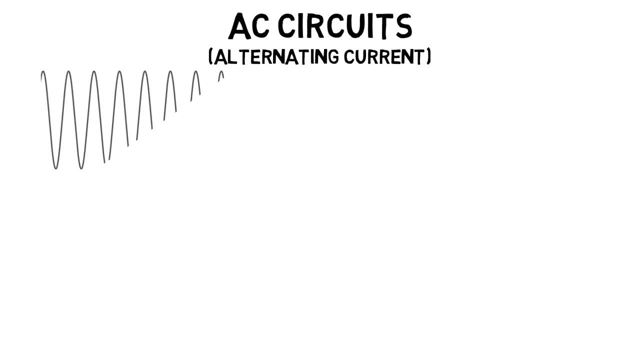 input voltage is no longer constant but sinusoidal and changing over time. For these circuits there's some more complexity added. Where a capacitor or inductor in a circuit with a resistor causes the voltage to change its amplitude but also shifts it, The capacitor or inductor can change the 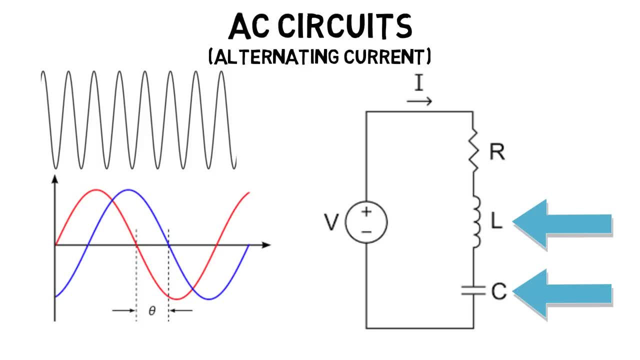 phase of the voltage within the circuit. The math behind this actually involves imaginary numbers. That square root of negative 1 you learned in high school actually has a ton of applications, and this is one. And it's not because current or voltage are imaginary, but using imaginary numbers just makes the math work when it comes to changing the phase or theta offset in a cosine or sine function. 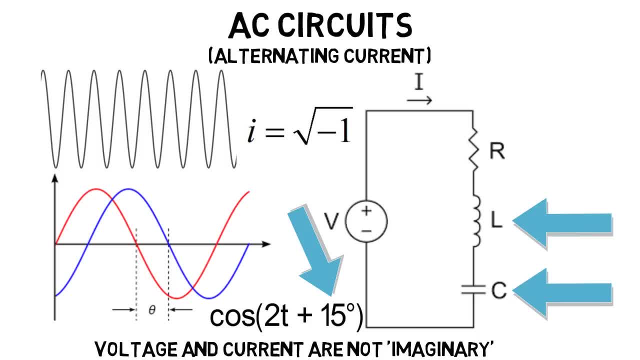 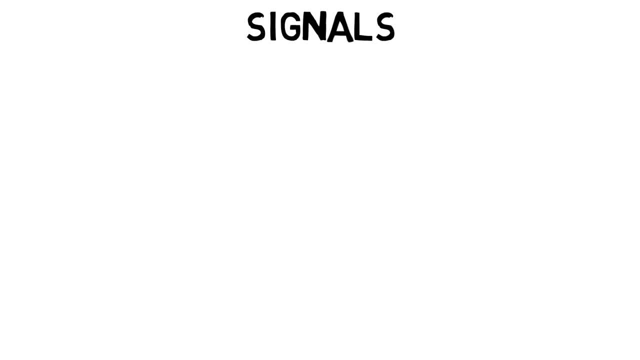 Don't worry about all that now, but it is something you will learn. There's, of course, plenty more in the basic circuits classes, but let's move on to the signals classes. These are essentially math classes and will be one of the most math intensive electrical engineering classes you'll take. Before this you've dealt with. 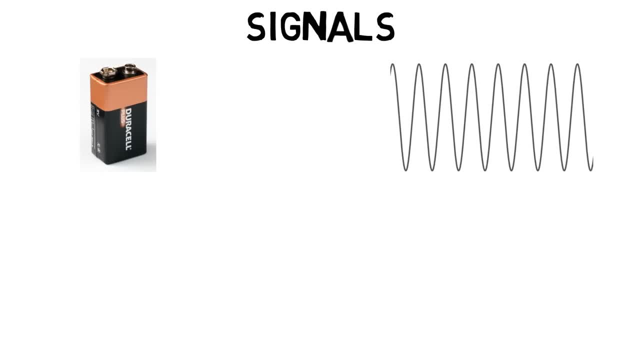 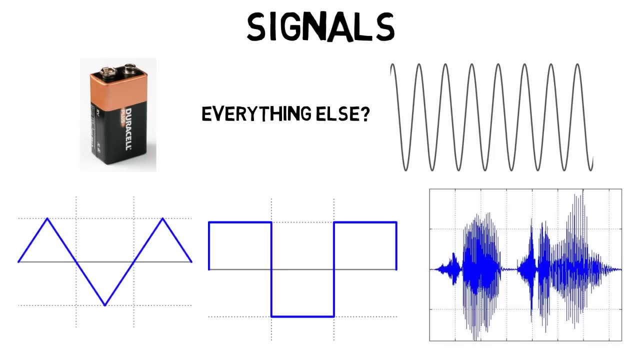 constant voltages and then sinusoidal voltages, but what about? well, everything else. You could have a triangle wave, a square wave or some really complicated and messy voltage, which is what real-world signals can be like. So what happens if you put those into a circuit? Well, in this first 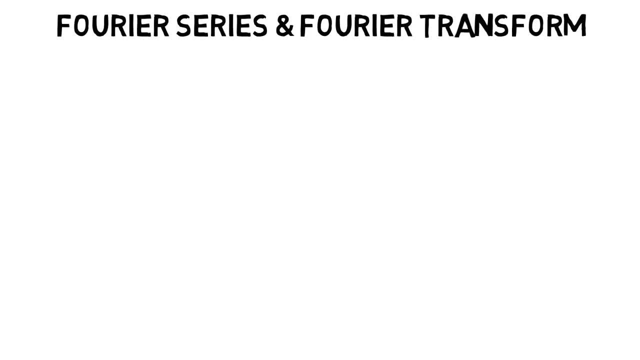 signals class you'll learn something called the Fourier series and Fourier transform, Something very important in physics, engineering and applied math. This says that any function can be made up of a bunch of cosine and or sine functions added up, often an infinite amount. Here we can see just a plain 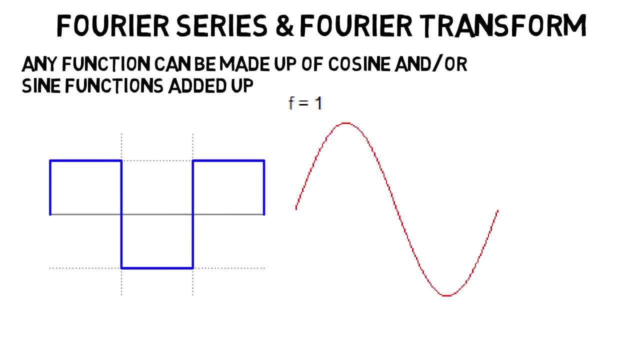 square wave. but if you have a sine wave and to another and then another, and you keep going picking sine waves, with the right amplitude and frequency, it will approach that square wave. In this class you will use some calculus and some new math concepts to find those frequencies and 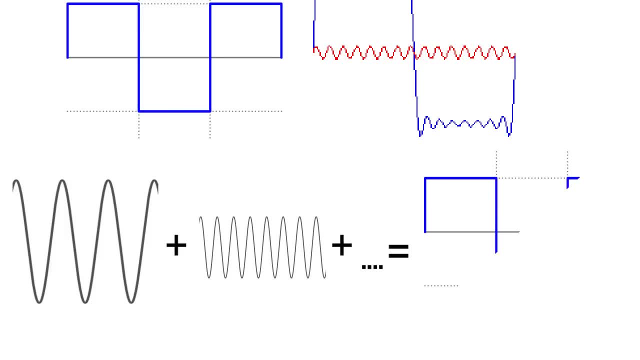 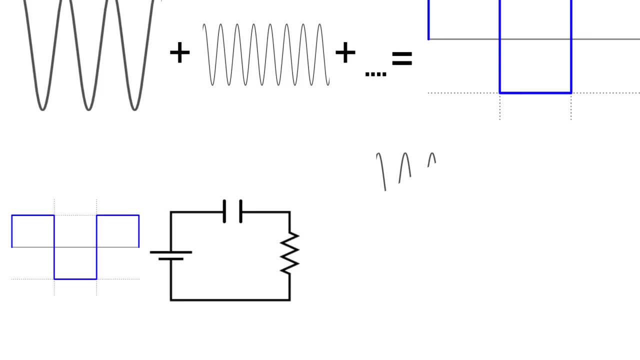 amplitudes of the sine functions that make up some other function. So now, if we put a square wave into the circuit and want to know what the voltage and current will look like, we can mathematically model it like putting in a bunch of sinusoidal waves of different amplitudes and frequencies, which you 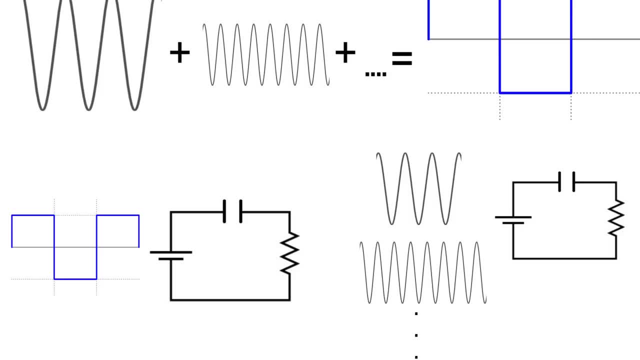 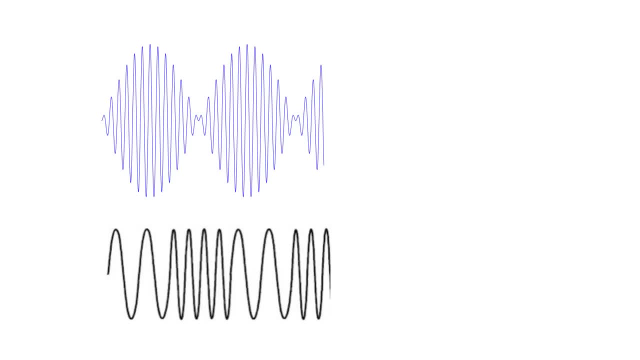 will already have under your bed. You'll learn lots of mathematical techniques to simplify this for you Now, two specific types of signals- you see here that kind of looks sinusoidal but not really- are AM and FM radio signals, which brings us to your wireless communications course. This class is not about physics, but just more of the math. 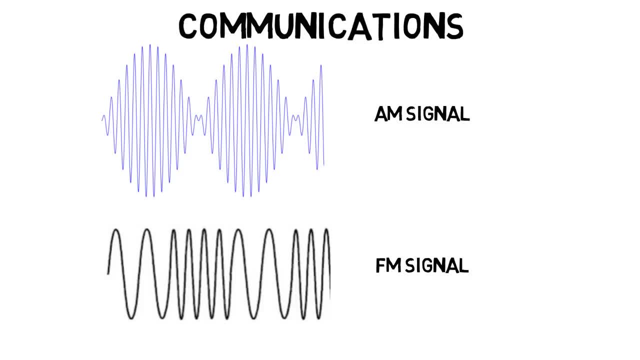 behind specifically AM and FM signals. If you look at a simple AM signal, you'll notice the amplitude oscillates up and down and if you look at an FM signal, the frequency oscillates throughout the wave. By making the signals look like this, it causes the frequencies to move up to some specific, unique. 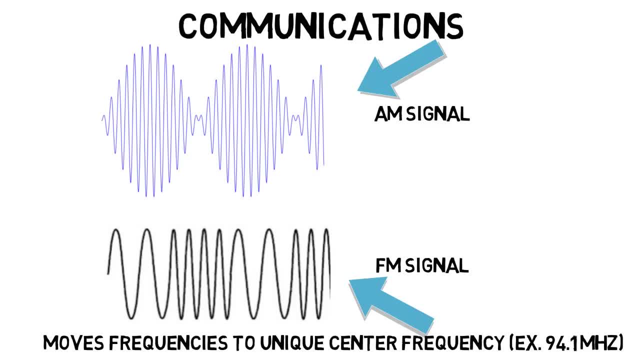 center frequency like 94.1 megahertz that the radio station transmits at. This is what the station 94.1 FM, is, Just that station transmitting at that specific frequency. Yes, it's more complicated, but that's the general idea Without that. 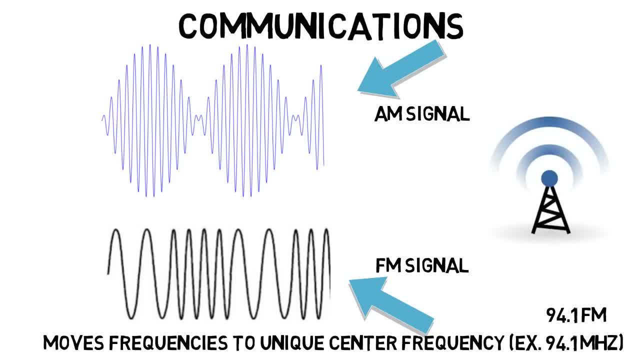 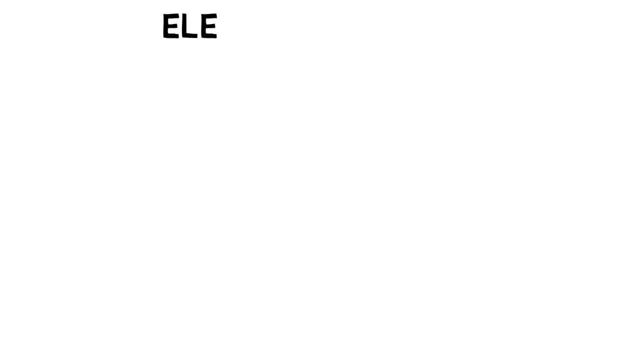 manipulation. you could not wirelessly send those signals for people to listen to in their cars. You'll learn why this has to be done and all the math behind that in this class. If you take your electromagnetism courses, it will be pretty much all. 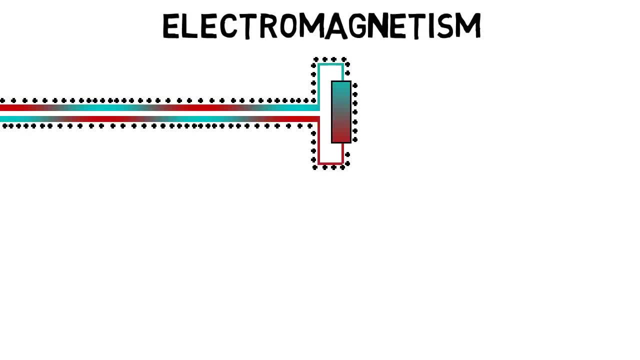 physics and involve a good amount of calculus. You'll see how, when you have a changing current, it creates a magnetic field around it, which then in turn creates an electric field around that, and this continues and this propagates as an electromagnetic wave, because it's electric and magnetic fields are coupled. 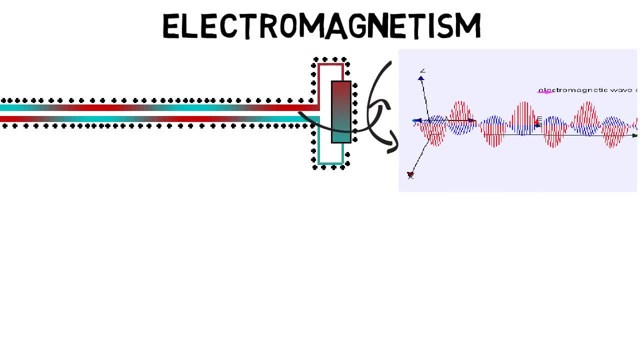 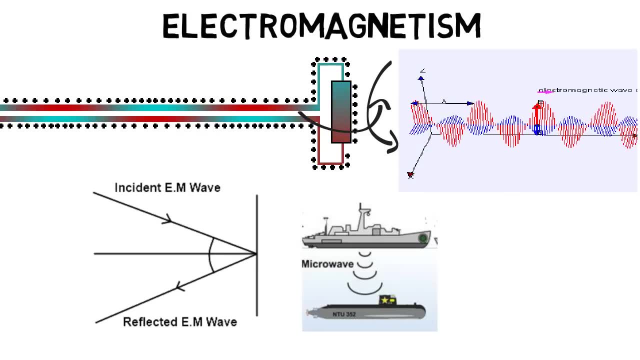 together You'll learn a lot about what those waves do when they interact with objects. like what if they hit some metal barrier or they encounter water? how far could they penetrate if there was a receiver at some depth? You'll also learn about transmission lines which aren't. 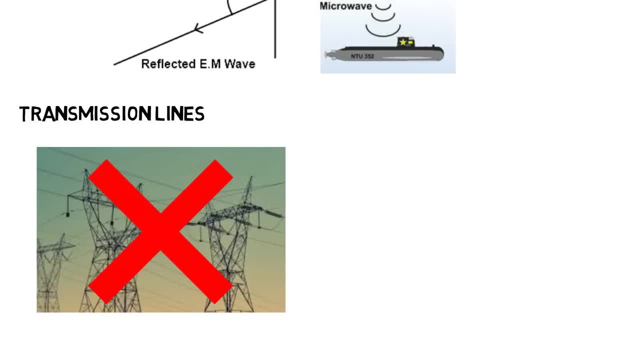 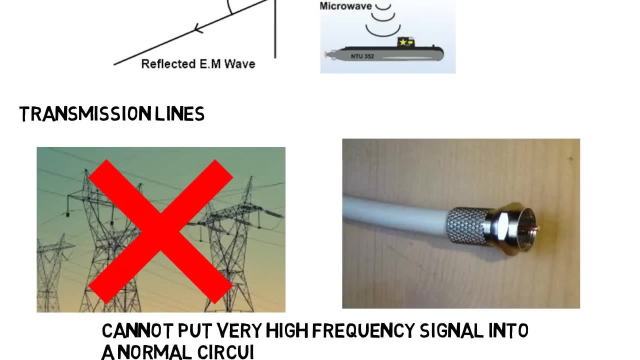 probably what you think of. The ones you learn in this class are cables that handle very high frequency signals that oscillate back and forth very quickly. You cannot just put a very high frequency signal into a normal circuit. Issues come up simply due to the laws of physics, and you'll learn about all that. 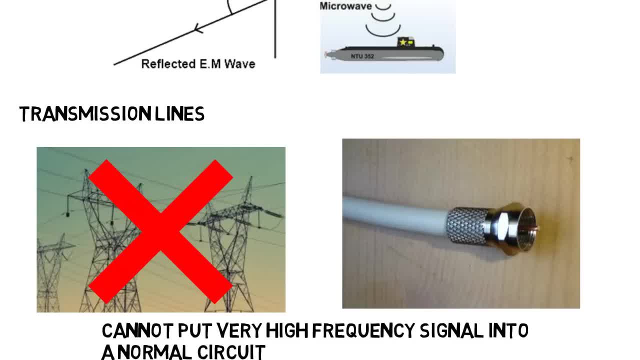 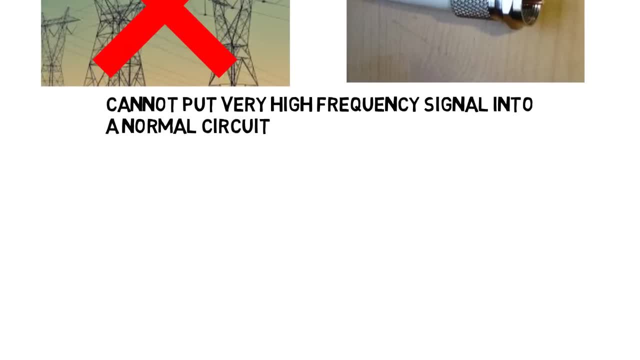 as well. Many of your other classes tell you about how to analyze signals and manipulate them for various purposes, but this class really teaches you about the physics of the waves, so you can understand things like how a wireless signal will be affected as it travels through Earth's atmosphere. when we have 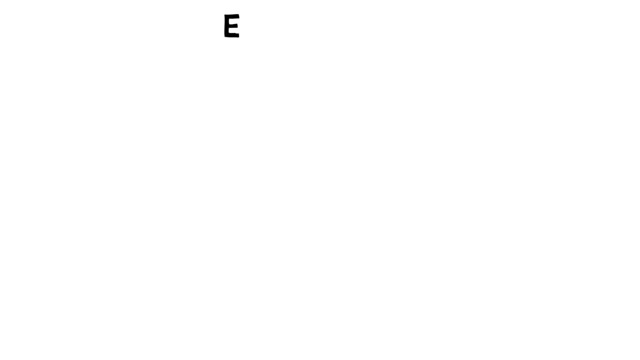 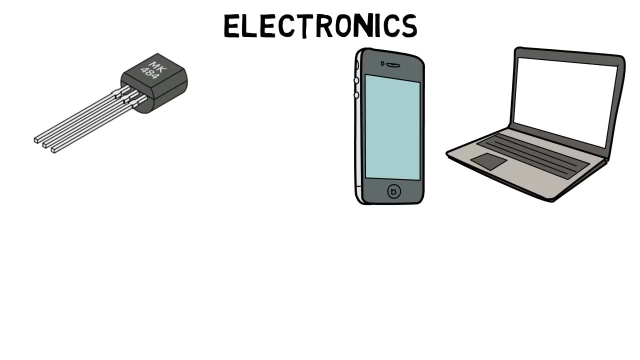 to communicate with a satellite, for example. Then, moving on in your electronics classes, you'll finally learn about the transistor. There are billions of these in your laptop and millions in your phone. to make them work, There are lots of kinds of transistors, but to simplify, 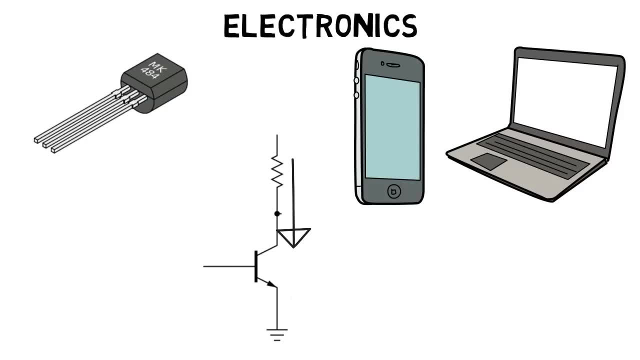 in a circuit. the current often flows down here and a little flows in here and they combine and flow out. here You'll learn more circuit analysis techniques to analyze voltage and current in these circuits, as always. but the thing is, by changing this voltage on the transistor you can control how much. 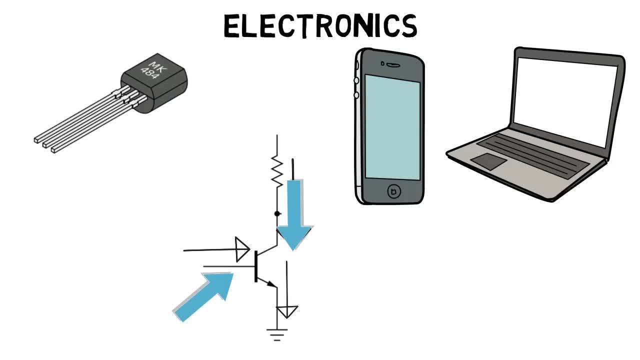 current flows through the transistor, Meaning the transistor can essentially act as a switch. It can allow current to flow, which is basically like the transistor being on, and it can shut off current flow, which is it being off. of course, This can create a high voltage. 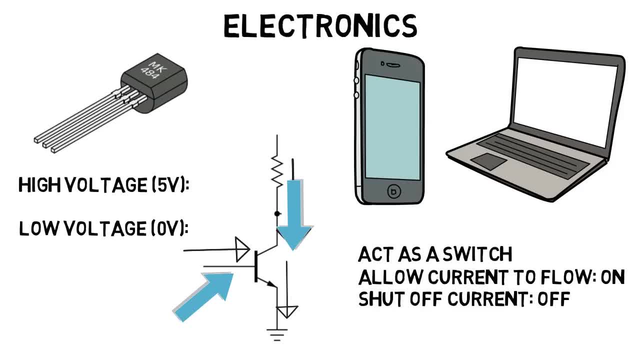 like five volts and change it to a low voltage like zero volts. This is the binary, or ones and zeros that are really under the hood of your computer. You will learn about making circuits that can switch quickly and efficiently in your digital electronics class. Analog electronics is more about using 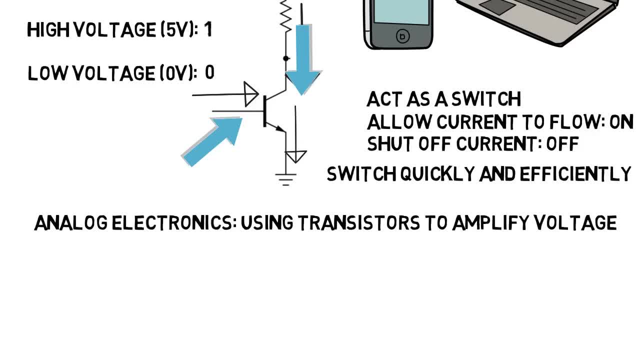 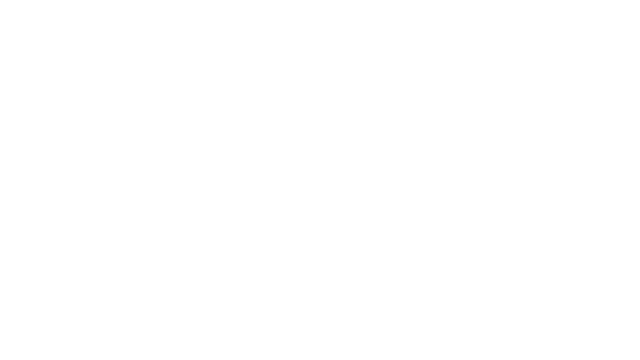 transistors to amplify a voltage, which is their other main application, where some of the same power sources can be needed to amplify a voltage. If this happens, we'll learn about principle amplification would, of course, be needed for music or hearing aids, as an example. 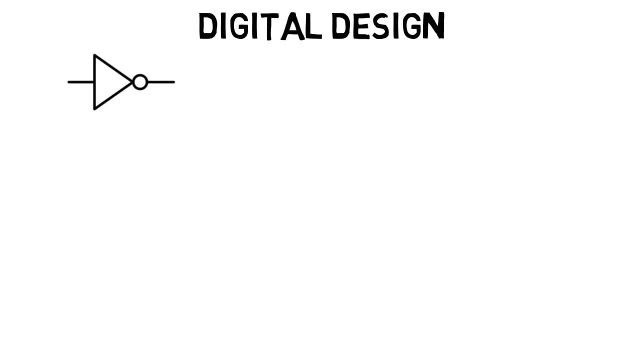 Now there are, of course, a few more classes I won't go into as much detail on. like in digital design, you learn about logic gates which take ones and zeros as inputs and output ones and zeros as well. The different gates output different things based on the inputs. Zooming into these is what digital electronics is. 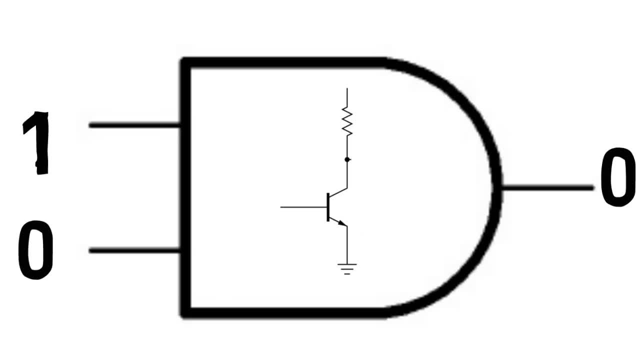 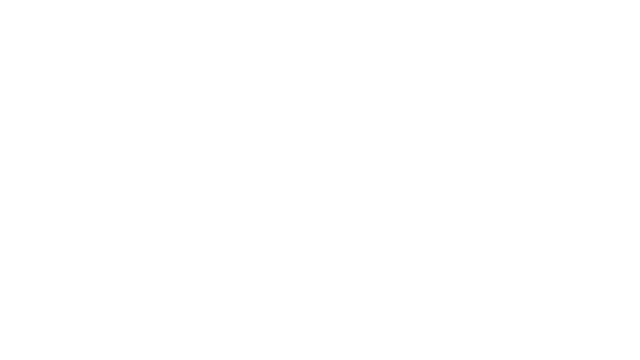 where you see the circuits that convert the high voltages to low voltages or vice versa. but in this class it's zoomed out, looking at the ones and zeros and making circuits with these logic gates. In the power electronics class we'll learn about the power supply. The power supply is a kind of a 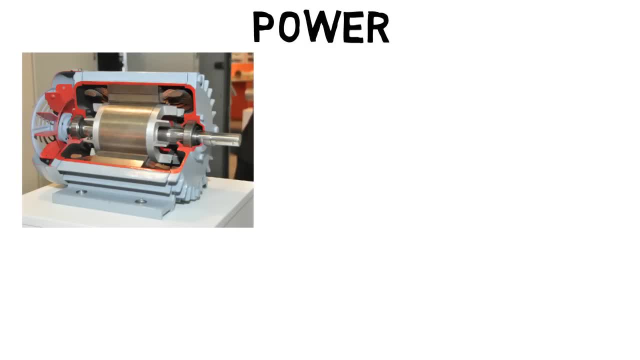 class. you'll analyze electric motors and generators and do circuit analysis with those. you'll do labs where you work with much higher voltages than normal, like over 100 volts. you'll see how much power is dissipated in resistor networks and so on. and the controls class has to do mainly with. 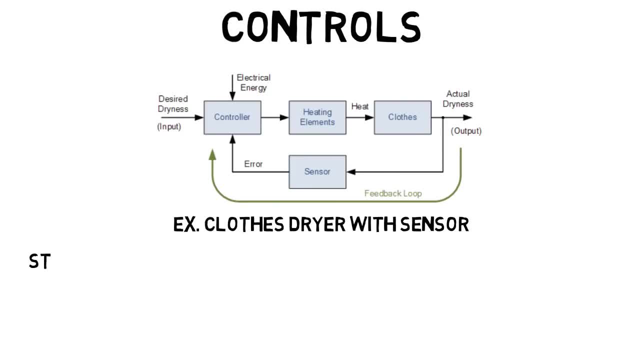 systems that involve some sort of feedback. you'll look at things like stability, because if you're constantly feeding information back into your system and something goes wrong, it could continuously be maybe amplifying some output, which will lead to issues. you'll also see a lot of these graphs. 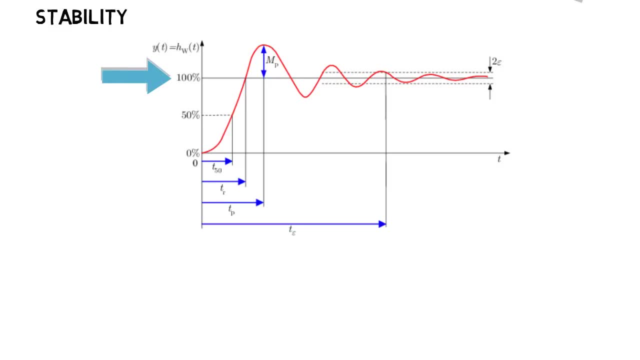 where you have some target output signal and in some cases there will be overshoot and then the signal will settle back to that target after a certain amount of time, versus just slowly charging up. you'll mathematically find that overshoot, how to minimize it or avoid it and, more hopefully, that